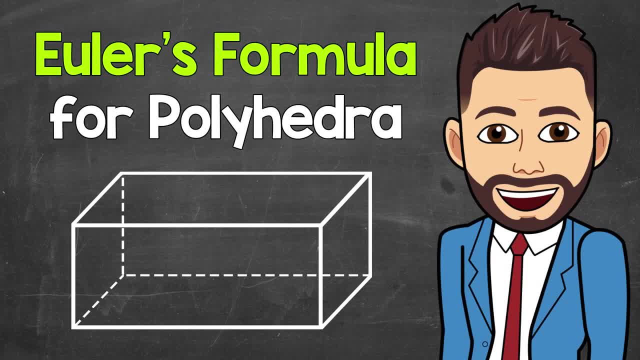 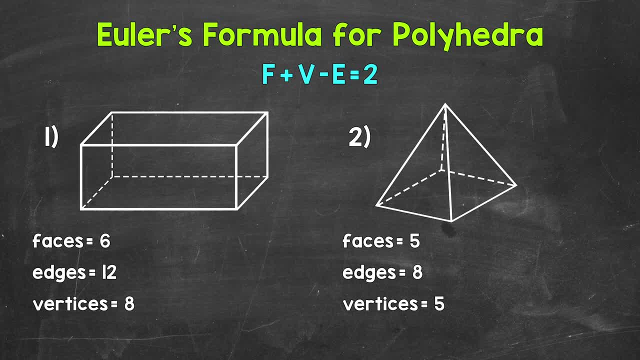 Welcome to Math with Mr J. In this video, I'm going to cover the basics of Euler's formula for polyhedra and what it is Now. basically, a mathematician named Leonard Euler figured out that there is a relationship between the number of faces, vertices and edges of a polyhedron, Simply put, the sum of the number. 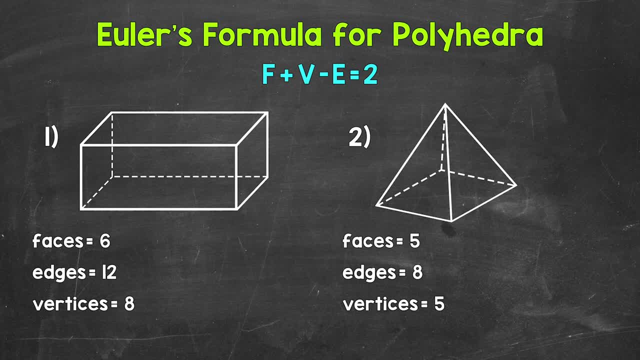 of faces and the number of vertices. so the number of faces plus the number of vertices is going to be two more than the number of edges. We can write this out as the number of faces plus the number of vertices, minus the number of edges, equals two. Let's go through a couple of 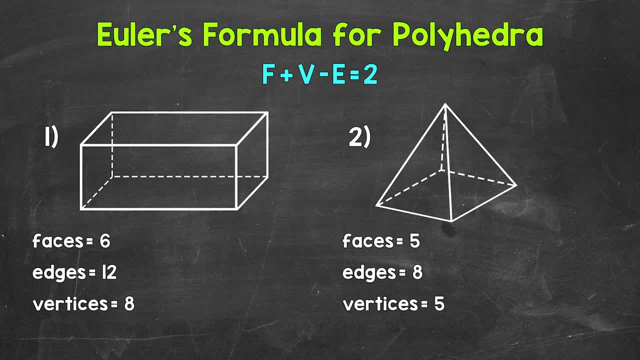 examples and plug in the number of faces, vertices and edges To show that the equation, this formula and this relationship is true. Starting with number one, where we have a rectangular prism, We have six faces, twelve edges and eight vertices. Let's 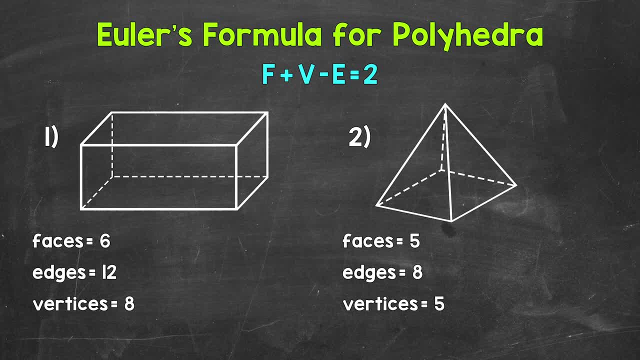 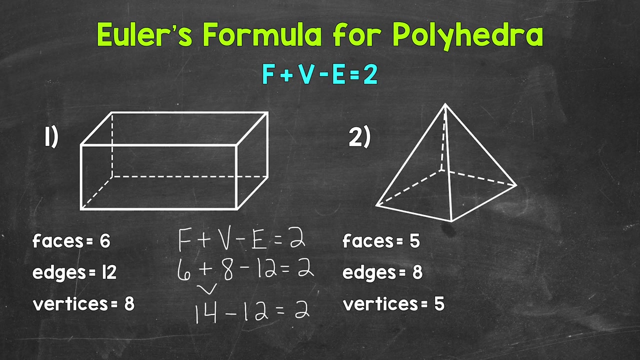 plug those into the formula to verify that they are correct. So the number of faces plus the number of vertices minus the number of edges equals two. So six faces plus eight vertices minus twelve edges equals two. Six plus eight equals fourteen. and then fourteen minus twelve gives us two. 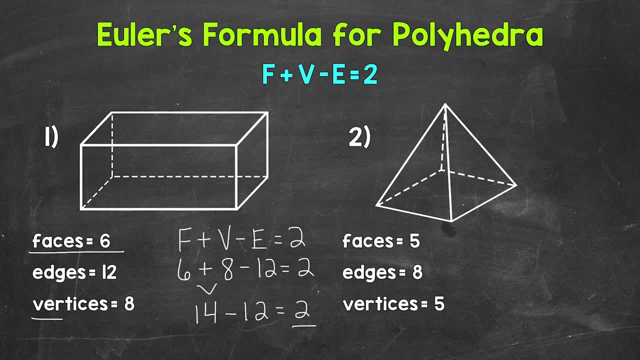 So if we take a look at the number of faces and the number of vertices, six plus eight that gives us fourteen. That's two more than the number of edges. let's move on to number two and try another example. we have a square pyramid for number two. so five faces, eight edges and five vertices. so the number. 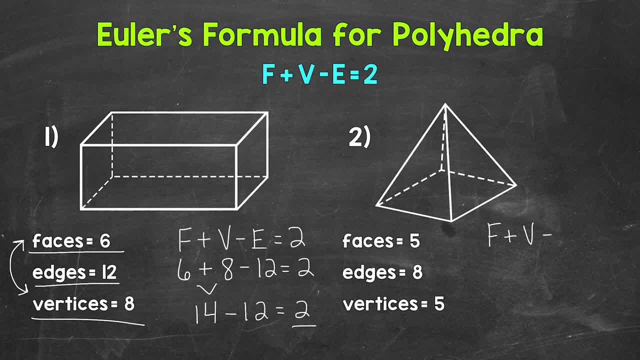 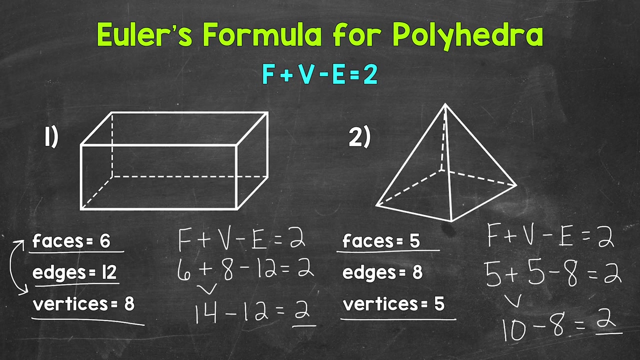 of faces plus the number of vertices minus the number of edges equals two. five faces plus five vertices minus eight edges equals two. five plus five is ten, minus eight is two. there are five faces and five vertices, so if we combine those we get ten, which is two. 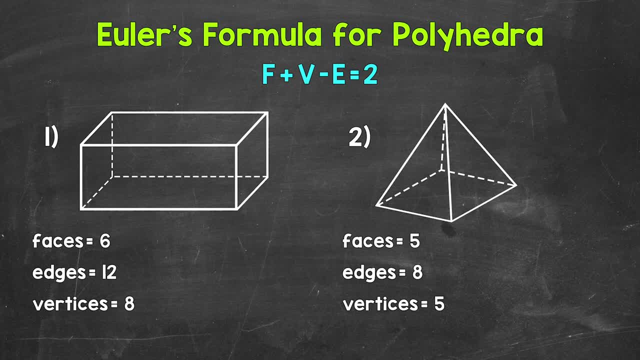 of faces and the number of vertices. so the number of faces plus the number of vertices is going to be two more than the number of edges. We can write this out as the number of faces plus the number of vertices, minus the number of edges, equals two. Let's go through a couple of 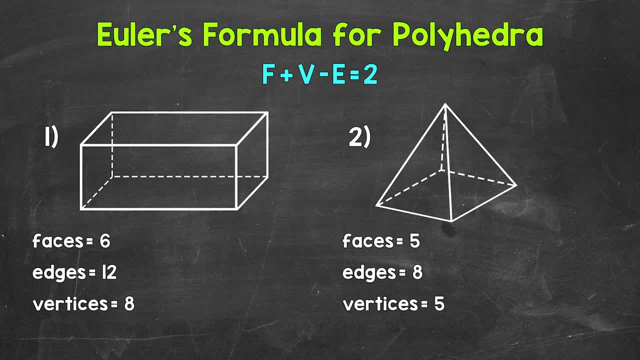 examples and plug in the number of faces, vertices and edges To show that the equation, this formula and this relationship is true. Starting with number one, where we have a rectangular prism, We have six faces, twelve edges and eight vertices. Let's 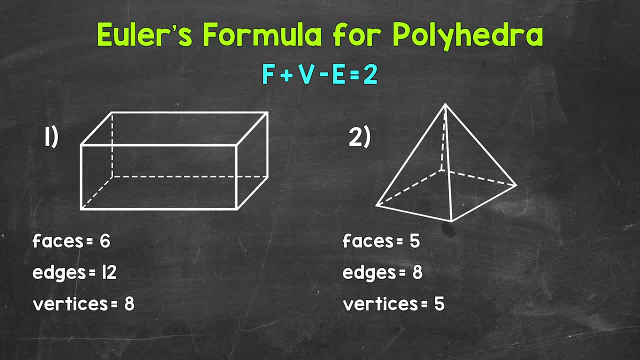 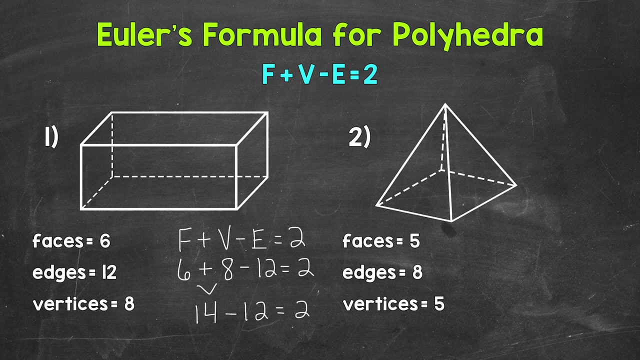 plug those into the formula to verify that they are correct. So the number of faces plus the number of vertices, minus the number of edges, equals two. To show that the equation, this formula and this number of faces plus the number of edges are correct, Let's plug those into the formula to verify that they are correct. Six faces plus the number. 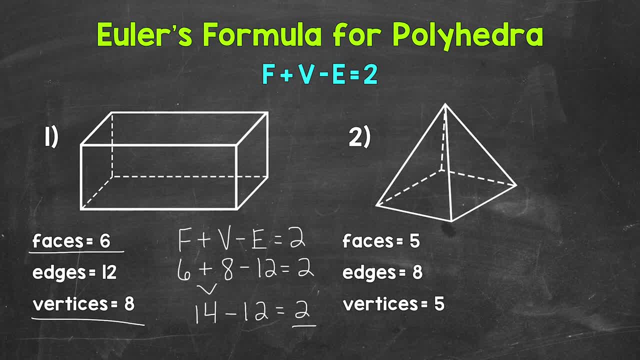 of faces plus the number of edges equals two. Six plus eight equals fourteen. and then fourteen minus twelve gives us two. So if we take a look at the number of faces and the number of vertices, six plus eight, that gives us fourteenthat's two more. 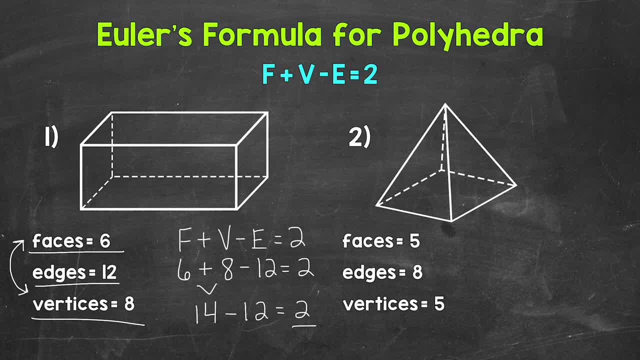 than the number of edges. Let's move on to number two and try another example. We have a square pyramid for number two, So five faces, eight edges and five vertices. So the number of faces plus the number of vertices, minus the number of edges, equals two. 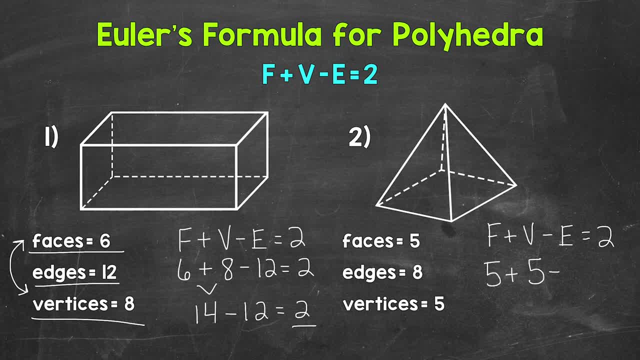 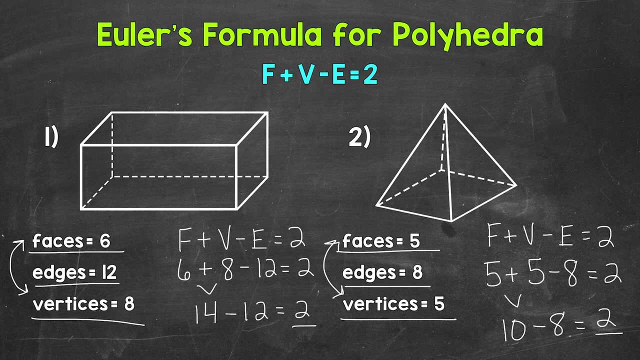 Five faces plus five vertices minus eight edges equals two. Five plus five is 10, minus eight is two. There are five faces and five vertices. So if we combine those, we get 10, which is two more than eight edges. So there you have it. 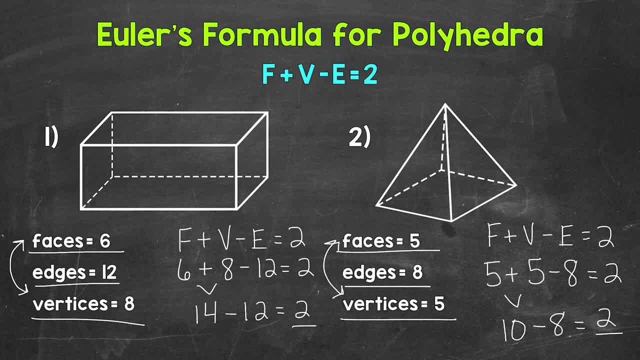 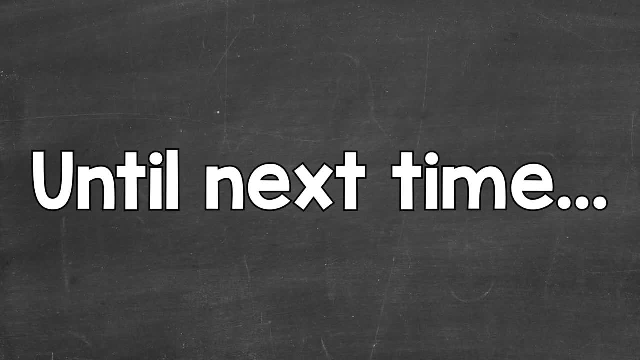 There is a basic explanation of Euler's formula for polyhedra. I hope that helped. Thanks so much for watching. Until next time, Peace.